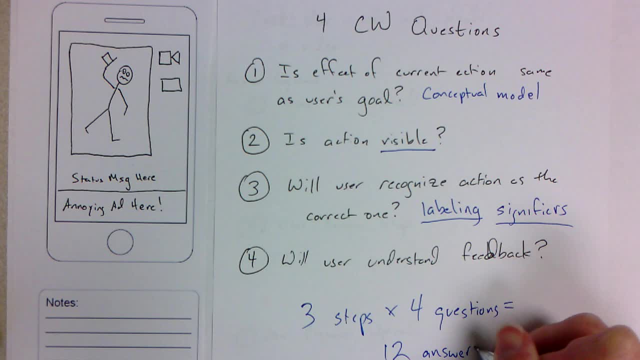 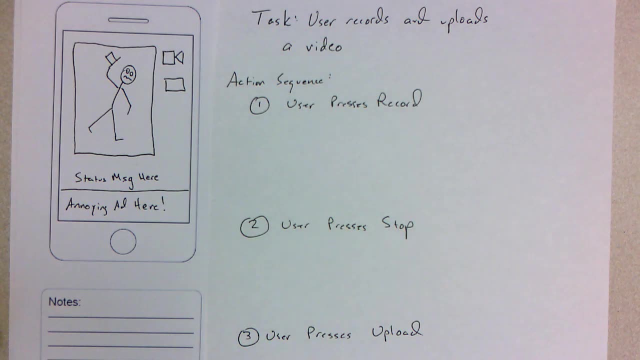 So that means, for this cognitive walkthrough we're going to write down 12 answers. So, without further ado, for the first step we're going to say, okay, the user's going to press record. So then at first we ask: okay, is that in line with the mental model? And yes, if you're going to record a video, you need to start. 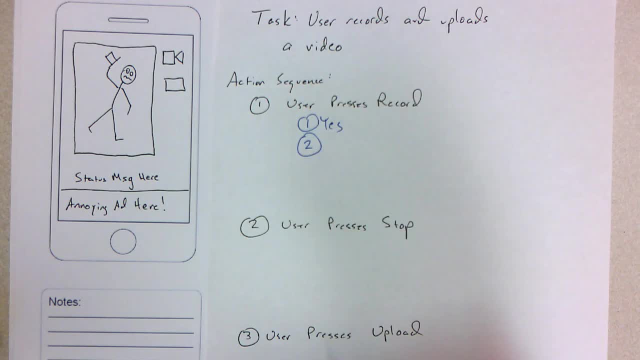 So for question one, we're going to answer yes. For question two: is the action visible? Well, it's right there. Yes. For question three: will the user recognize the action as the correct one? Well, this becomes a little bit tough. This depends on the user. 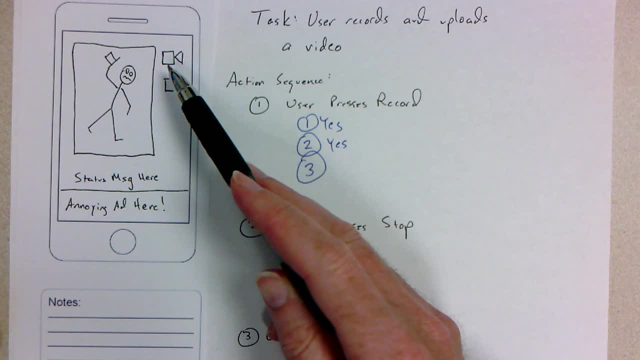 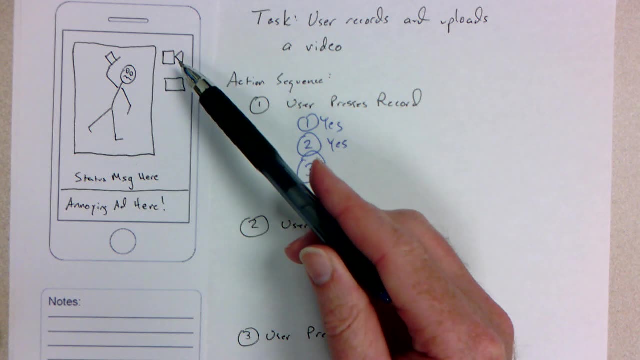 This is an icon pretty much just taken straight from a lot of iPhone apps, So the answer may be yes, but if we have particularly novice users, if we have young children, or if we have the elderly who are maybe new to smartphones, the answer might be no. 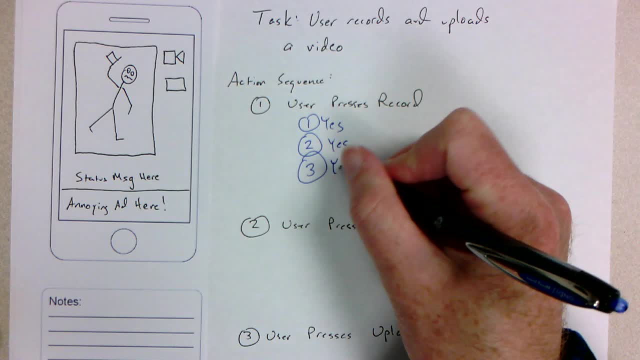 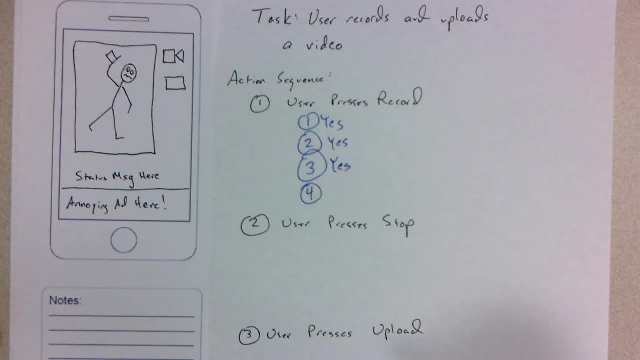 This is going to depend on our target users. Right now we'll say: our target user is your typical technology-savvy IUS student. so, yes, we'll give that a yes. When they start recording, will the user understand the feedback? 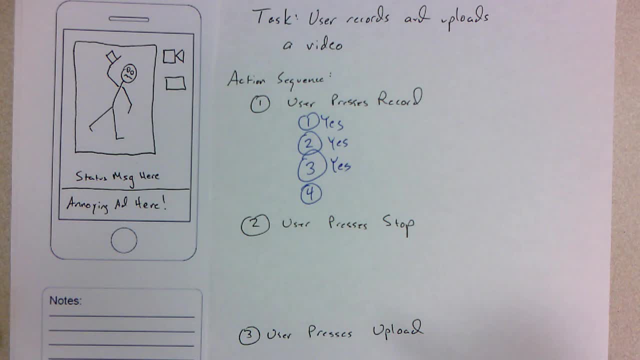 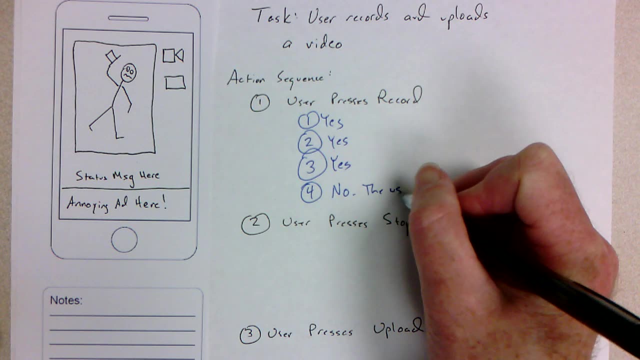 Yes, At this point we actually don't quite know, because we don't know what kind of feedback is going to happen, And so what we would write here is something like: maybe no, the user needs clear feedback And, even better, we can recommend what kind of feedback. 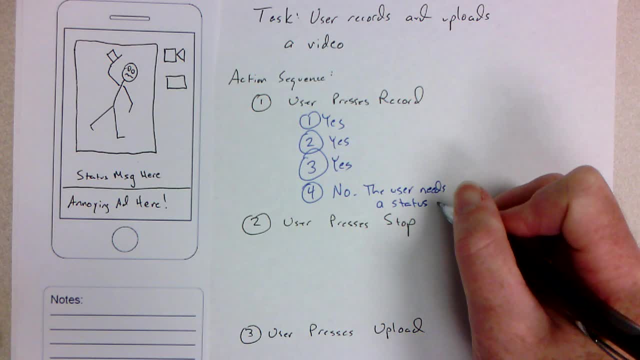 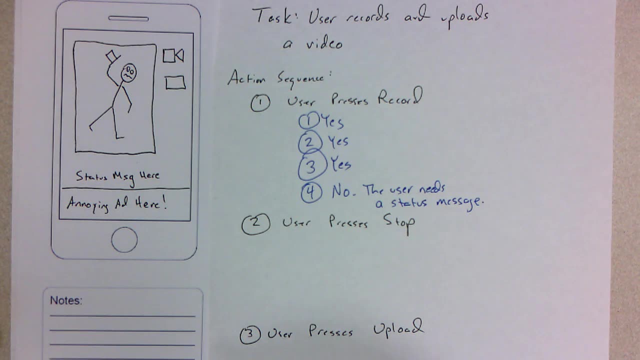 We can say the user needs a status message. That's not the only option. It could be that the stop button is grayed out so that the user can't use it until the record button has been pressed. So it could be that the stop button increases in visibility. 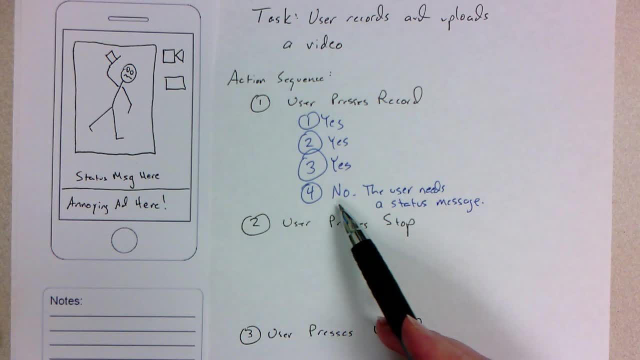 But for purposes of just making it clear we're not going to do that, For purposes of just illustrating the cognitive walkthrough: when we answer no, we make a recommendation to improve it. So then for the second one, the user presses stop. 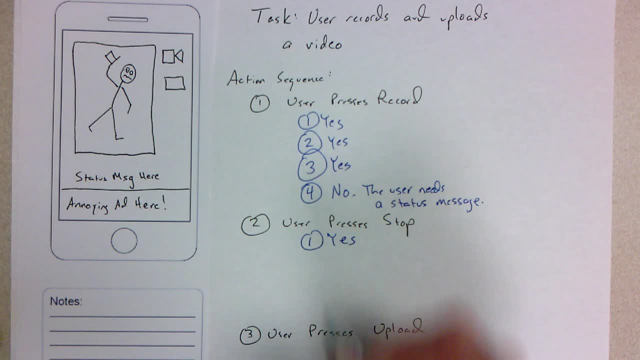 So question one: is that what the user wants to do? Yes, they're ready to stop recording. Is the action on the screen? Yes, it's a button right here. Will the user recognize the action as the correct one? Possibly, It's the universal symbol for stop. 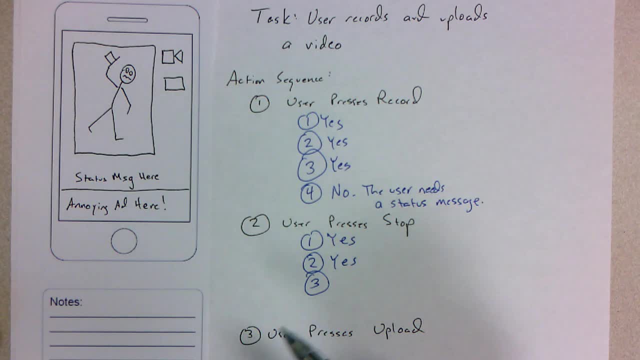 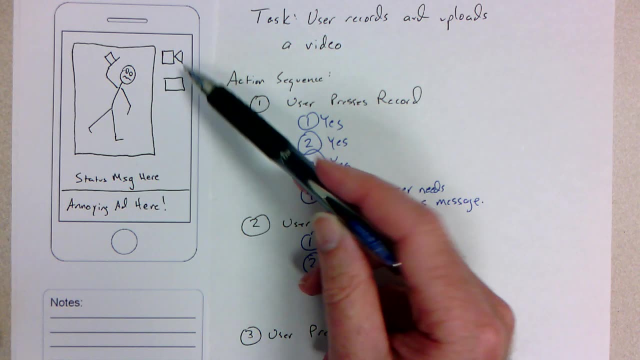 A lot of iPhone apps now use an X instead, And when we read about stop, we're going to use an X instead. And when we read about stop, we're going to use an X instead. And when we read about stop, we're going to use an X instead. 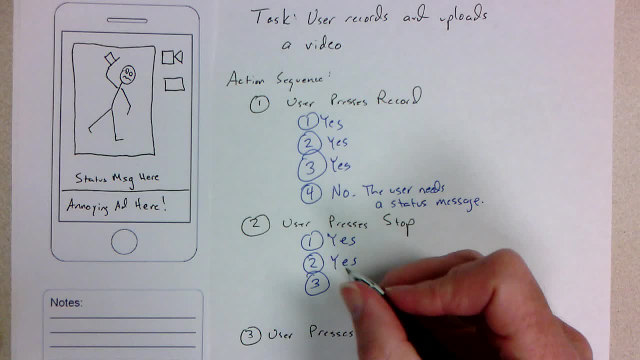 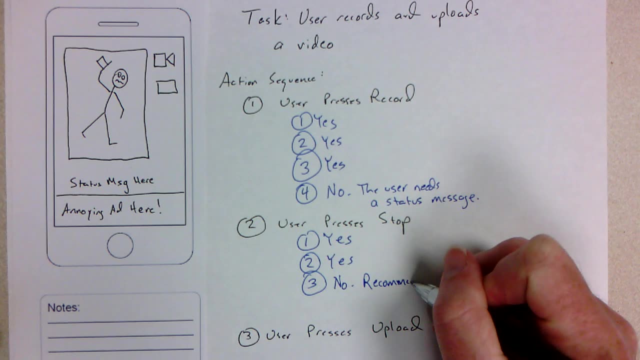 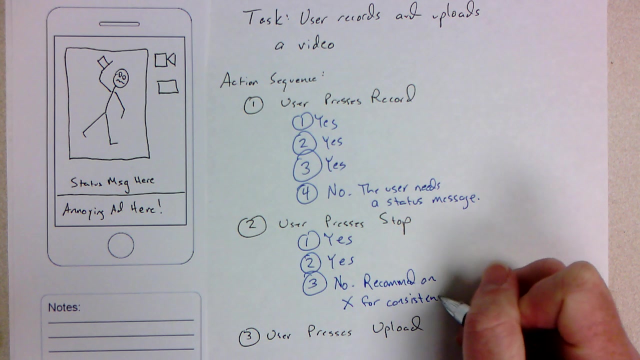 So we might want to recommend another symbol. So what we can say here is: maybe no, they won't recommend using an X instead. So what we're striving for here is consistency with other iPhone icons in this case. So what we're striving for here is consistency with other iPhone icons in this case. 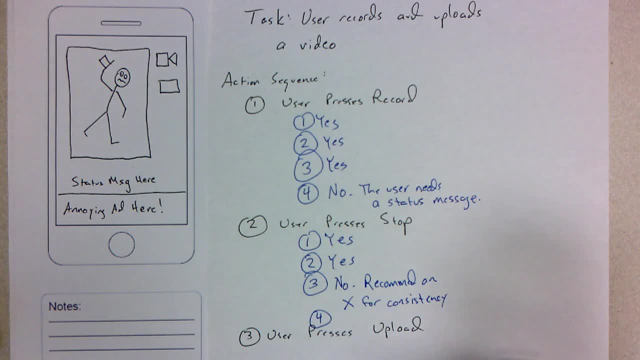 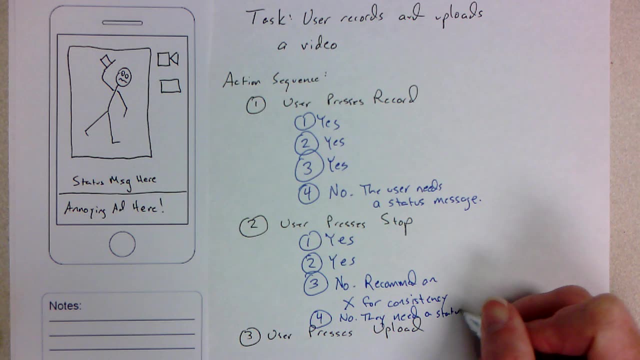 Finally, will the user understand the feedback they get? Well, we would say the same as for no, they need a status message. So the reason we don't know what kind of status message the user is going to get, even though it says on our prototype status message, goes here: 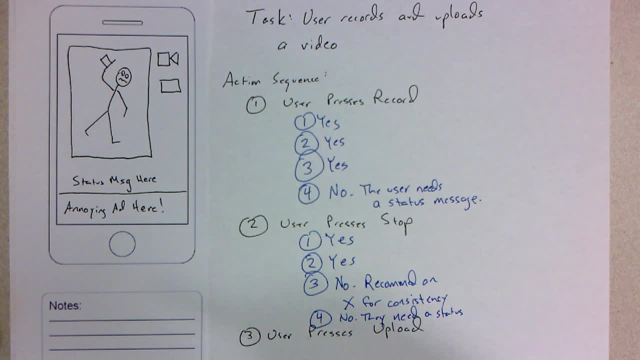 is that we don't have any annotations, We don't have any extra notes that tell us about that. So then the third step: the user is going to press the upload button, So I don't have room at the bottom of the page. 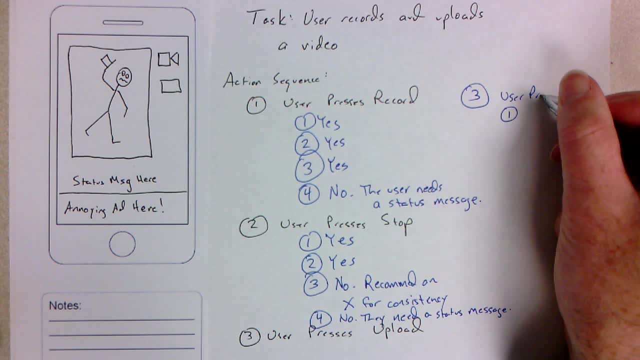 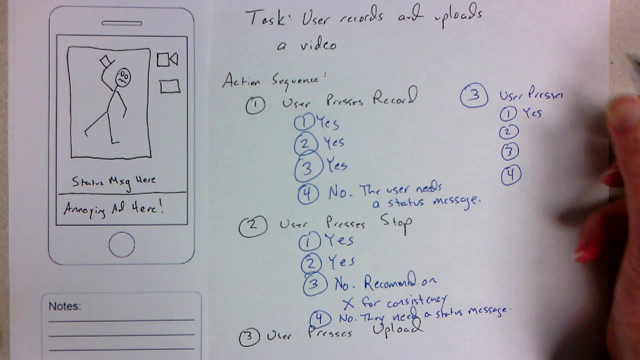 I'm going to answer those questions here. So the issue with this is we say: oh well, where's the upload button? So the mental model part is fine, The user wants to upload, It's time to do that, That's okay. 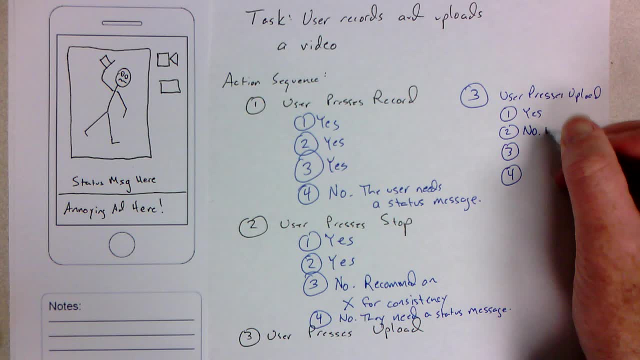 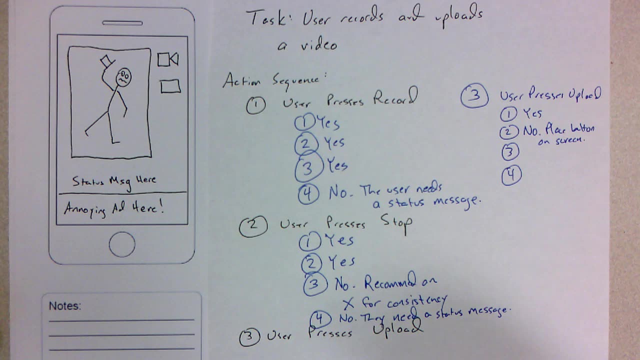 But the button is just not there, It's not visible. So we say no, place a button on the screen. Then, once we've written that, we have to answer the other questions as if everything is okay. So is the labeling okay. 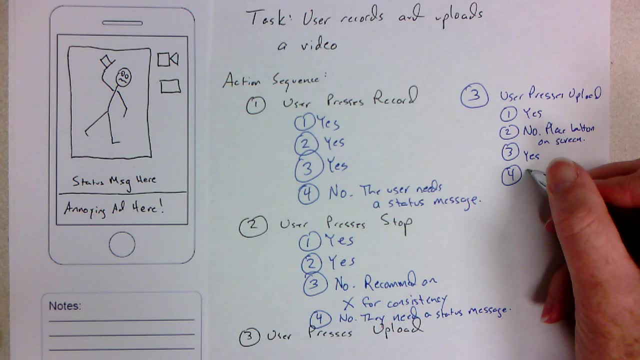 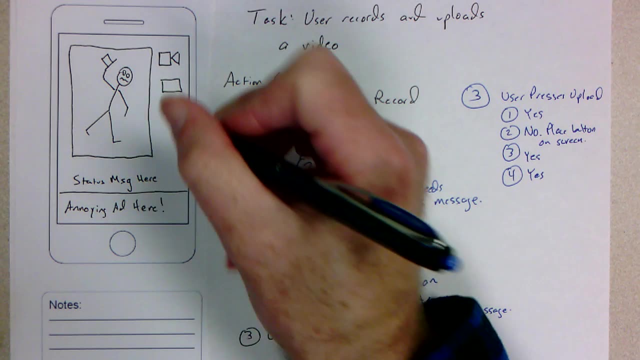 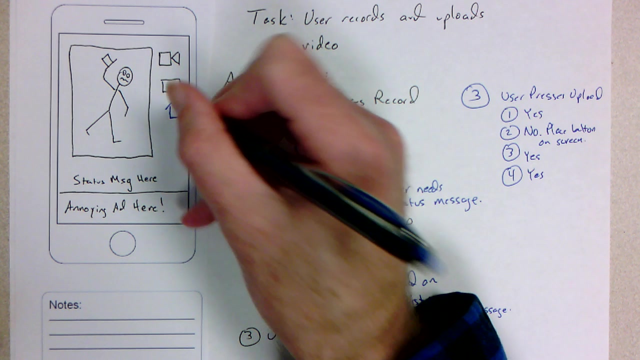 Yes, assuming that the button is adequate. that gets placed on the screen. Will the user understand the feedback? Yes, assuming they get feedback. So the button we would want to place on the screen would be something like: maybe it goes right here, Maybe it's our standard up arrow or one of these things that indicates share. 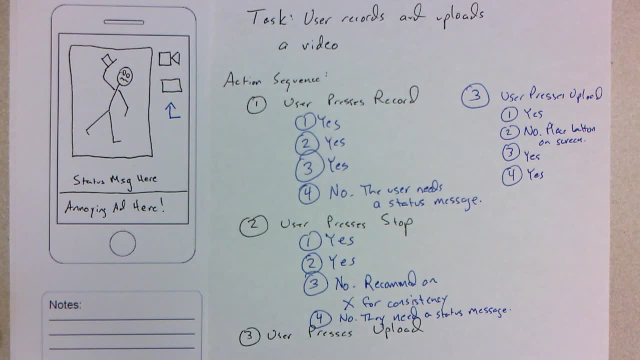 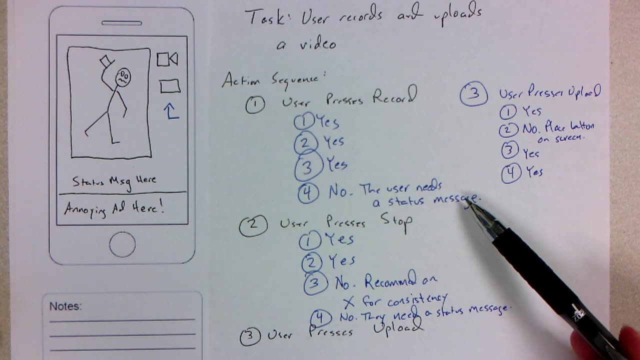 depending on the icons that we're using. So this is just a quick example of a cognitive walkthrough. We answer all the questions at every step. When we answer no, we make a recommendation. A lot of informaticists, a lot of HCI practitioners feel that.